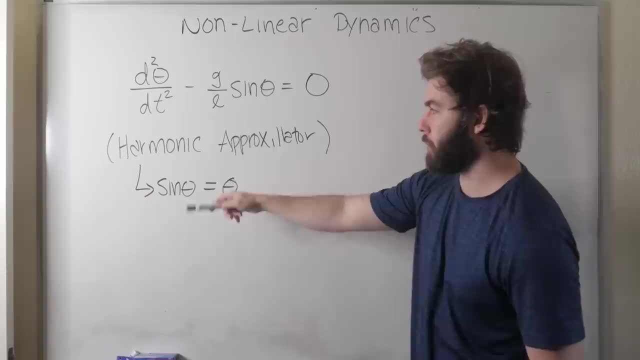 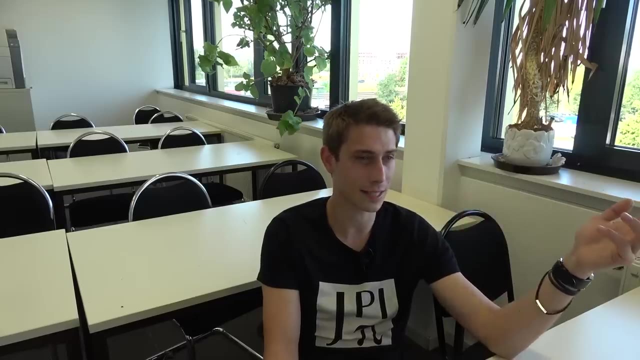 And by higher order I mean after the first term. So for the harmonic approximator we take sine of theta equal to theta. Yes, Andrew, Why are we even interested in something that we can't solve analytically? That's not even close to being rigorous, Mr Hilbert. 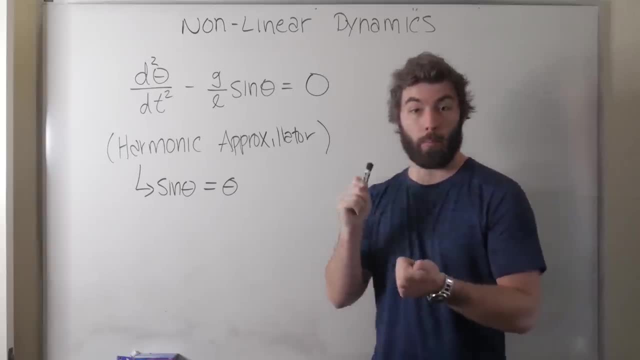 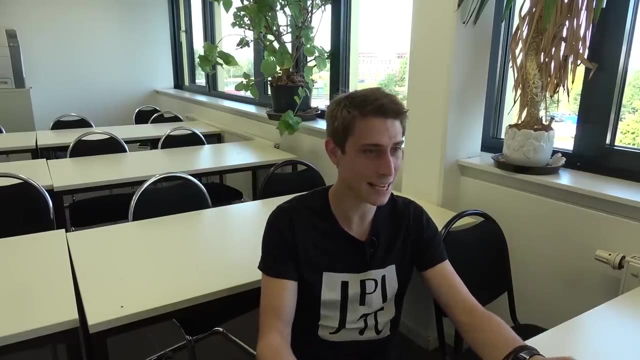 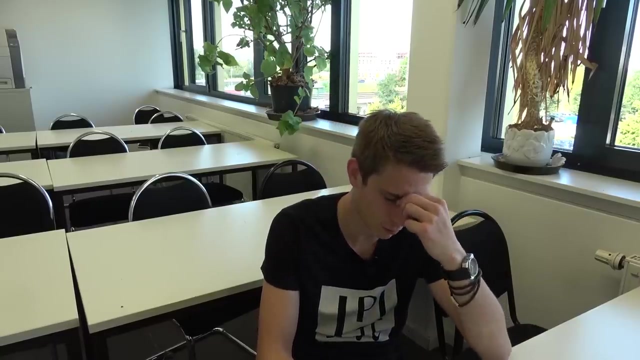 We're not here for rules, For rigor, Andrew. We're here to approximate and apply and then repeat. Why did I sign up for this course? then Wikipedia clearly stated that chaos theory and non-linear dynamics are a branch of mathematics. Once again, you fooled me, Wikipedia, just like with probability. 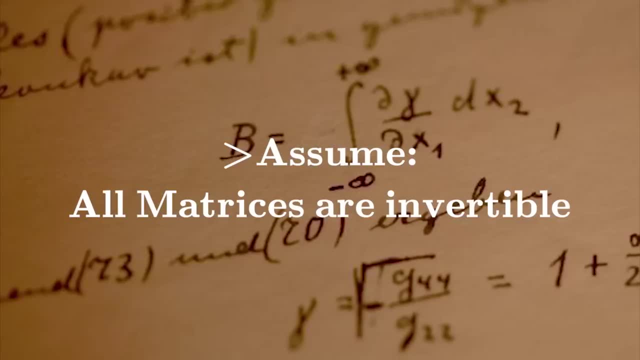 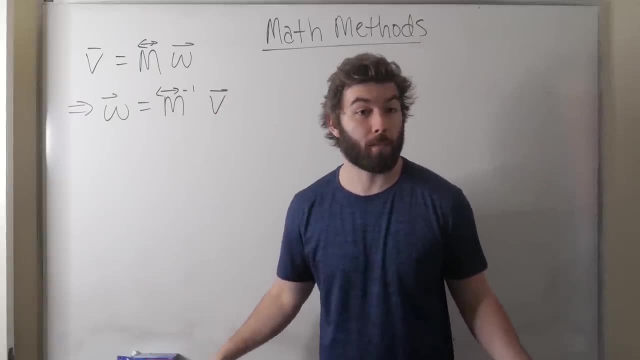 theory. A lot of systems in physics can be expressed in terms of matrices. If I poke a system, I want to know how it responds. But you can also ask the inverse question. If I have a response, what must the source have been? 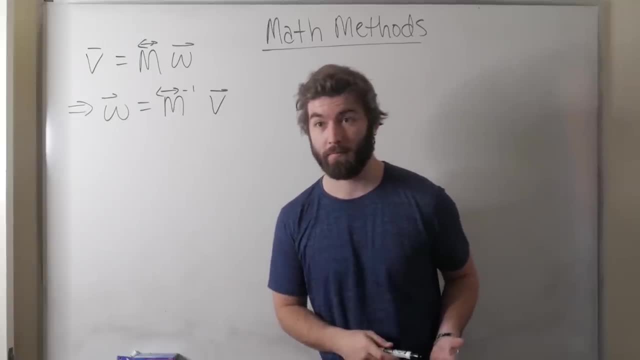 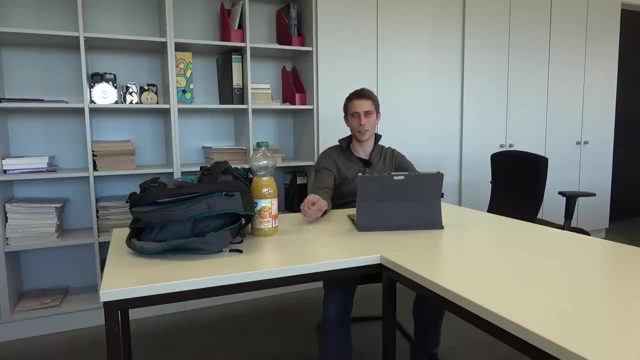 So I can always hit rewind by inverting the matrix. But, Mr Andrews, linear algebra tells us that we can only really have a real multiplicative inverse for square matrices, Square matrices With a non-zero determinant. Listen, if it's in physics it's invertible, But Mr Andrews, 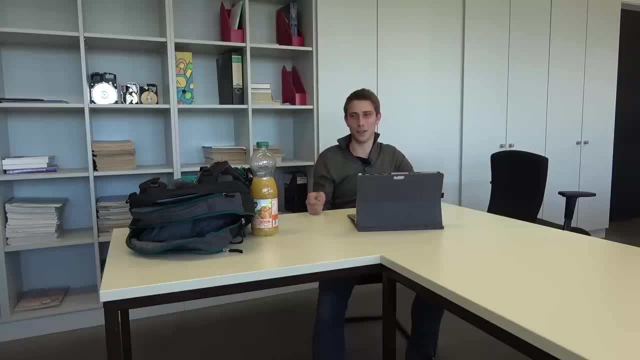 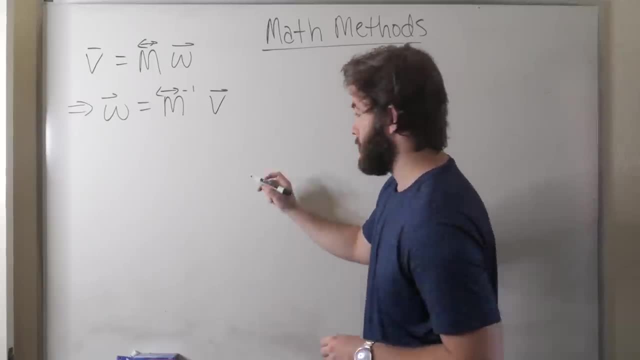 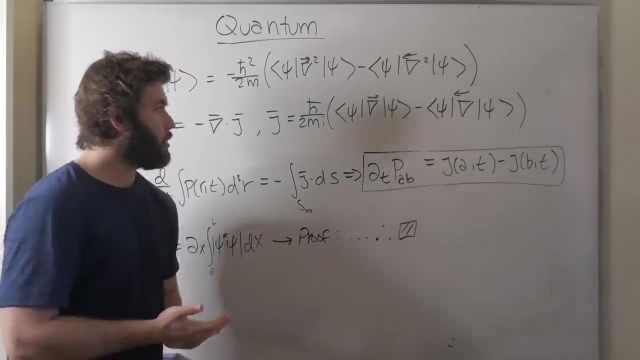 that's obviously wrong. You even wrote this as a theorem on the last blackboard. Anyways, let's do some examples. Let's consider a 3 by 2 matrix with real entries. We know to talk about probability in quantum mechanics. we have to specify an interval, And if we define the probability, 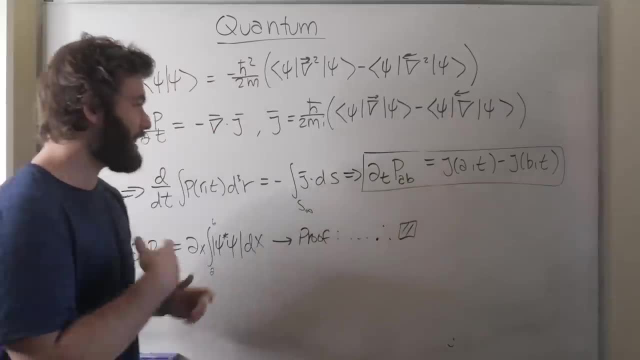 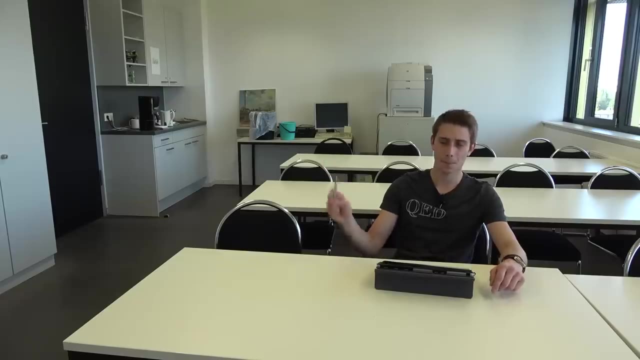 current. we can relate the two through this equation here, And in order to prove this, all you have to do is swap the integral with the derivative and go from there. It's very trivial stuff. But, Mr Medlet, you are assuming an interchange of limits, right there? 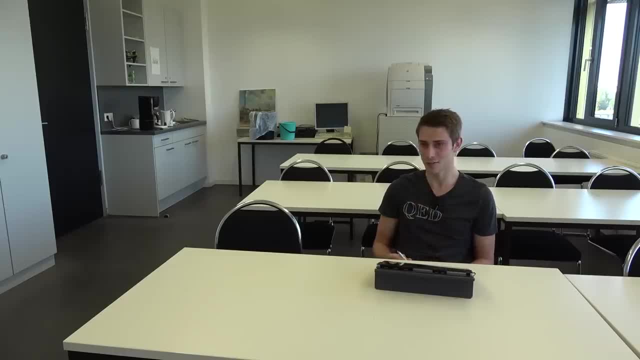 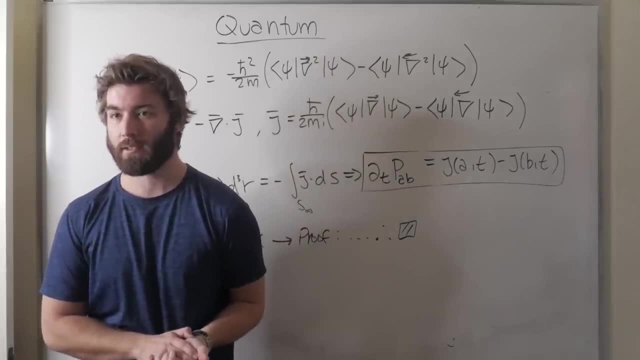 That's not a trivial thing. in the normal case, That even justified, does the integral even exist in the first place? Again, John, this is not a math class. I don't know why you insist on acting out. But, Mr Medlet, this is really important. 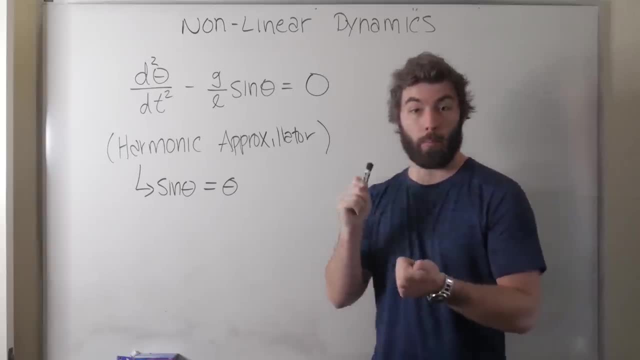 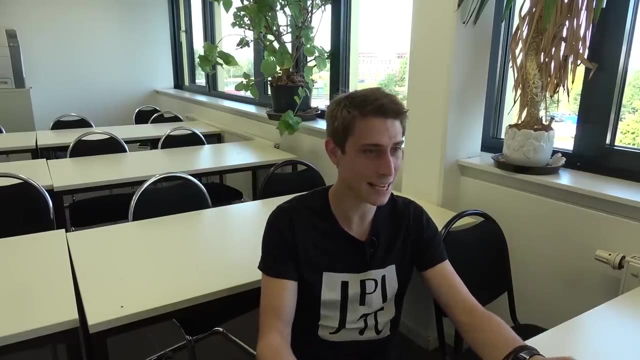 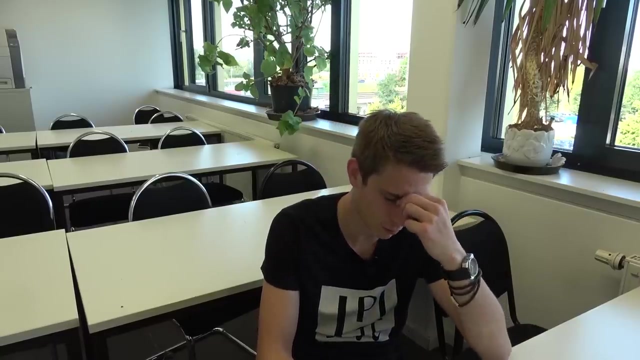 We're not here for rules, For rigor, Andrew. We're here to approximate and apply and then repeat. Why did I sign up for this course? then Wikipedia clearly stated that chaos theory and nonlinear dynamics are a branch of mathematics. Once again, you fooled me, Wikipedia, just like with probability. 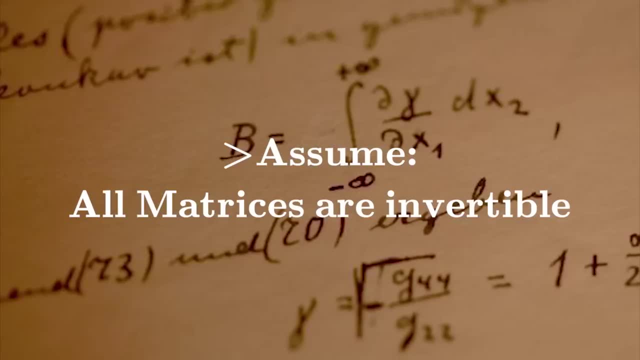 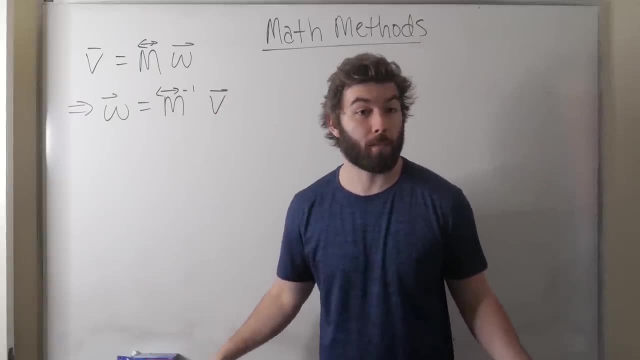 theory. A lot of systems in physics can be expressed in terms of matrices. If I poke a system, I want to know how it responds. But you can also ask the inverse question. If I have a response, what must the source have been? 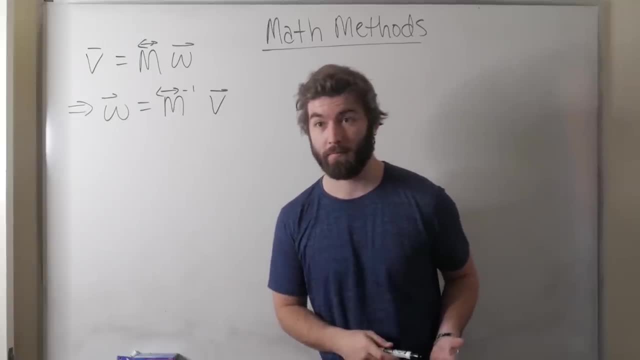 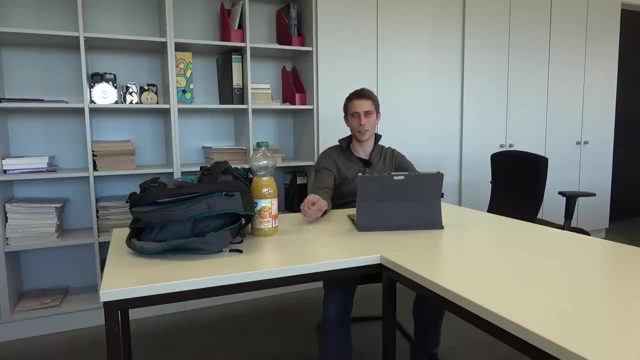 So I can always hit rewind by inverting the matrix. But, Mr Andrews, linear algebra tells us that we can only really have a real multiplicative inverse for square matrices, Square matrices With a non-zero determinant. Listen, if it's in physics it's invertible, But Mr Andrews, 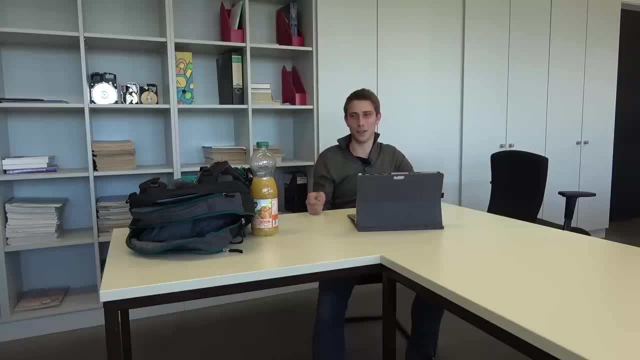 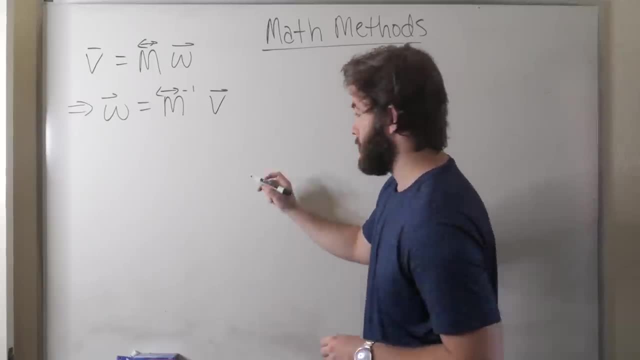 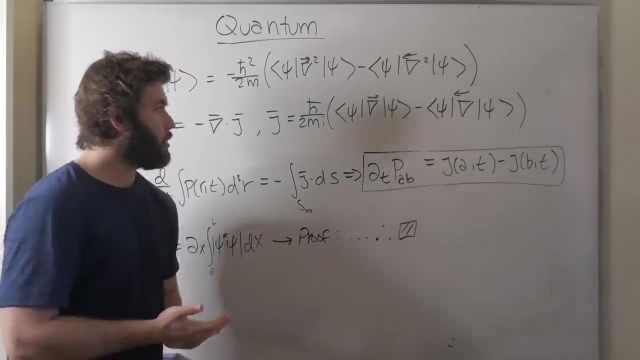 that's obviously wrong. You even wrote this as a theorem on the last blackboard. Anyways, let's do some examples. Let's consider a 3x2 matrix with real entries. We know to talk about probability in quantum mechanics. we have to specify an interval, And if we define the probability, 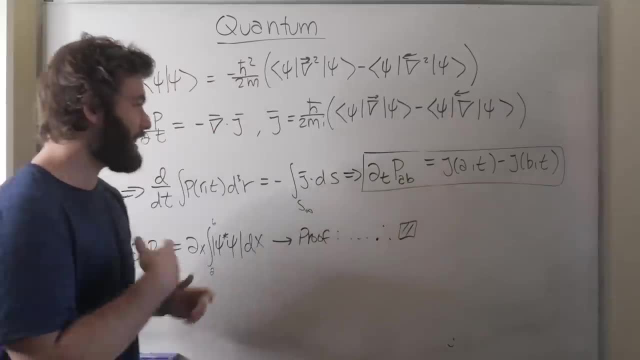 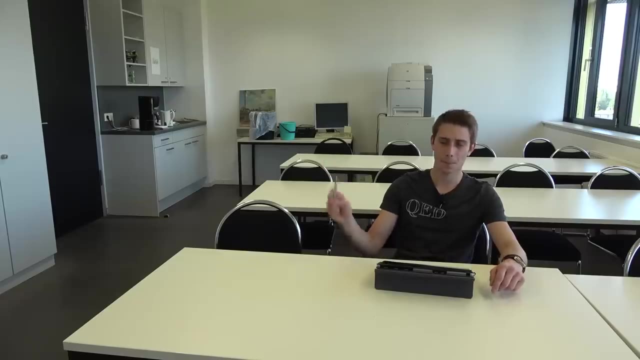 current. we can relate the two through this equation here, And in order to prove this, all you have to do is swap the integral with the derivative and go from there. It's very trivial stuff. But, Mr Medlet, you are assuming an interchange of limits, right there? 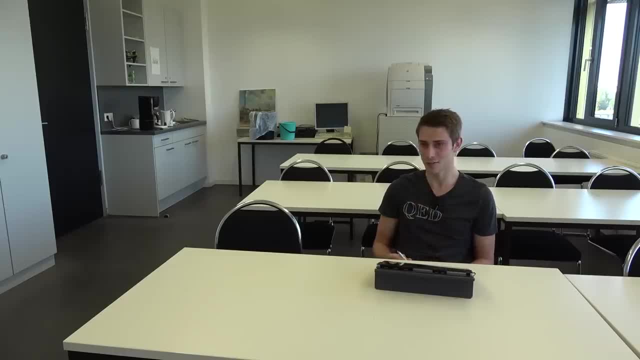 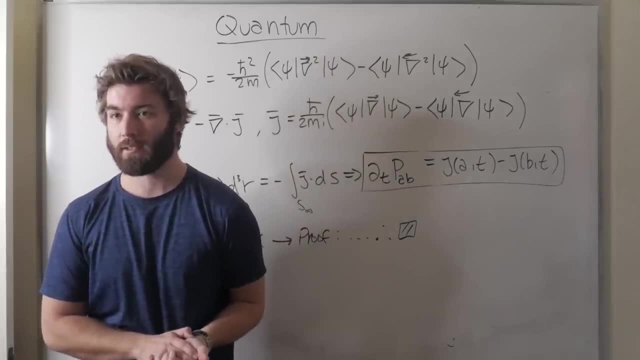 That's not a trivial thing. in the normal case, That even justified, does the integral even exist in the first place? Again, John, this is not a math class. I don't know why you insist on acting out. But, Mr Medlet, this is really important. 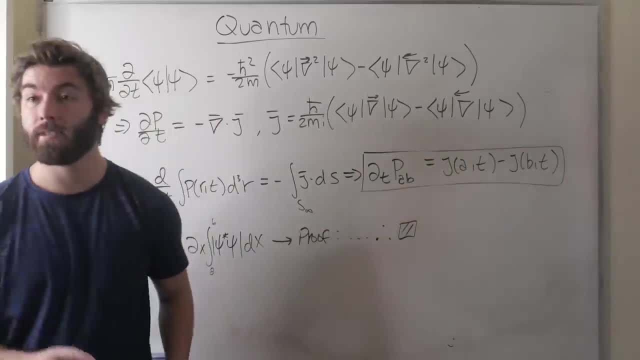 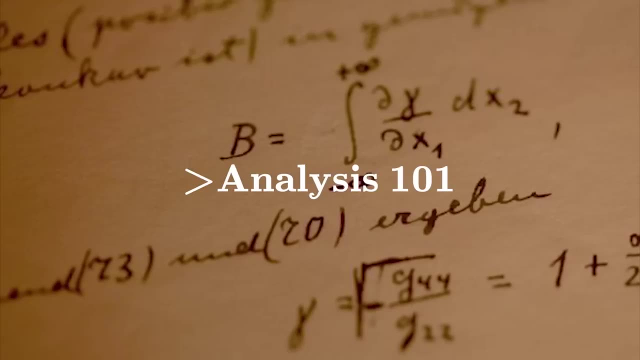 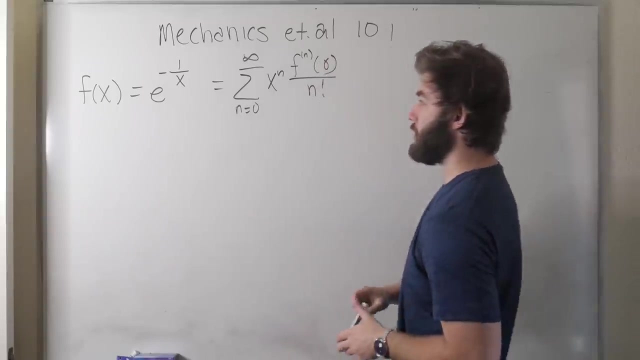 To me. Okay, enough is enough. See me after class and we can talk about the existence and probability of you flipping burgers for the rest of your life. So we need something to either drive or damp the system depending on x, which is the role of this function here, But instead of working with the exponential 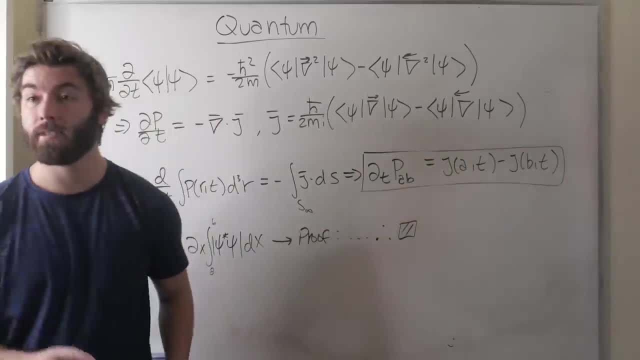 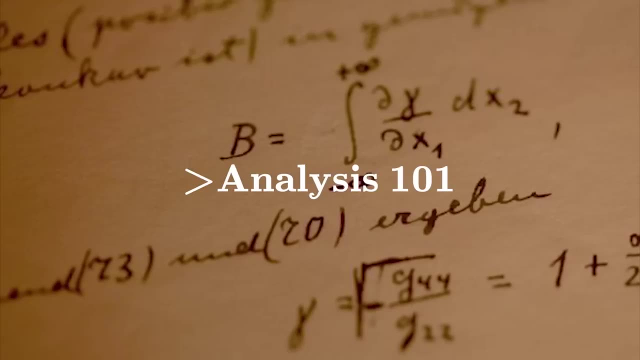 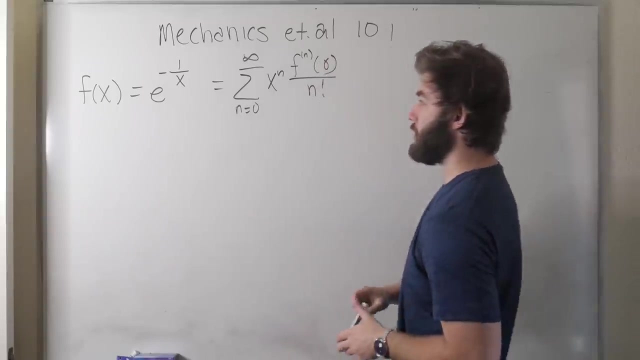 To me. Okay, enough is enough. See me after class and we can talk about the existence and probability of you flipping burgers for the rest of your life. So we need something to either drive or damp the system depending on x, which is the role of this function here, But instead of working with the exponential 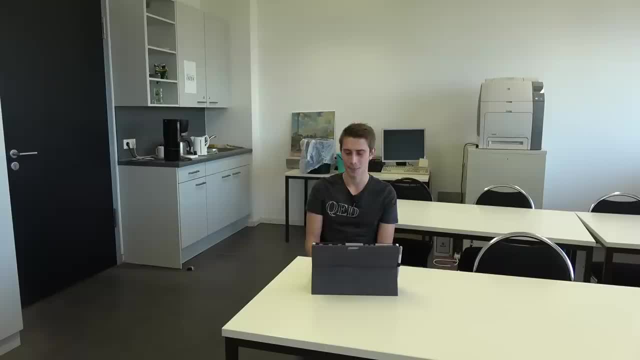 we're going to go ahead and expand it in a Taylor series centered at 0.. But, Professor Chattington, even though the function is infinitely often differentiable, I agree on that- It is not analytical Meaning. we cannot turn it into a Taylor series. 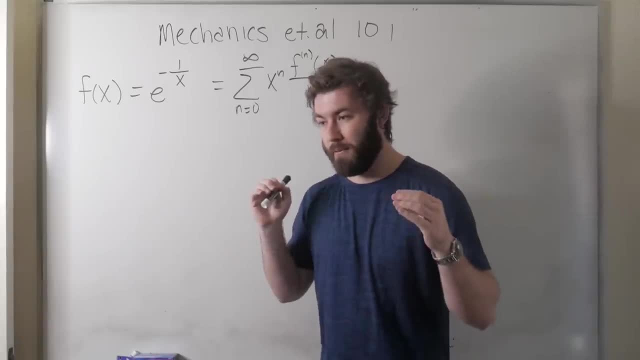 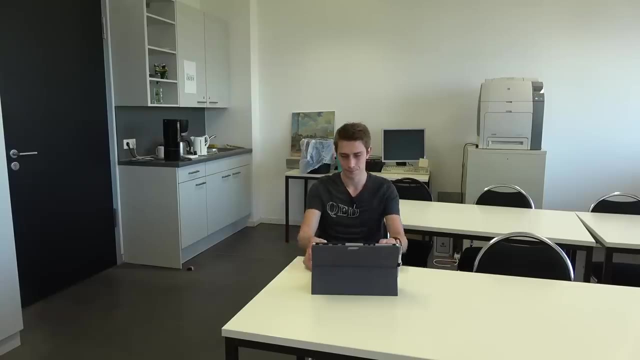 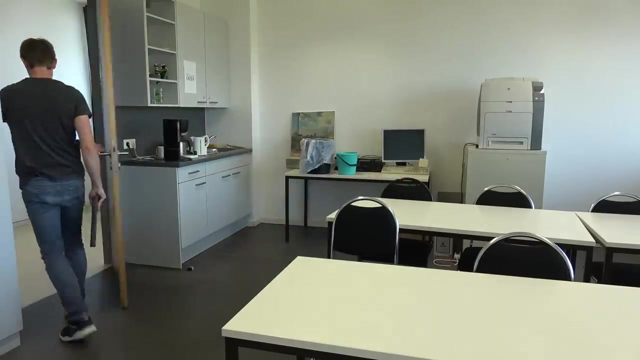 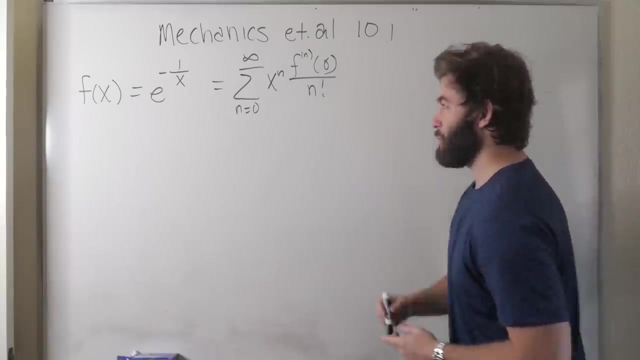 Even though it's infinitely differentiable. What are you even saying? Listen, if you have questions about the rigor of this class, you can leave. Please, Ait, I'm a head out. Okay, where were we? 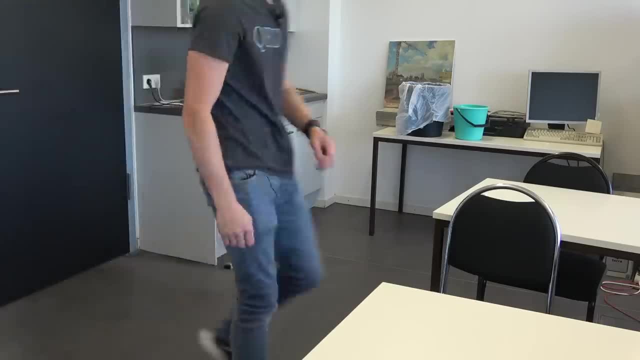 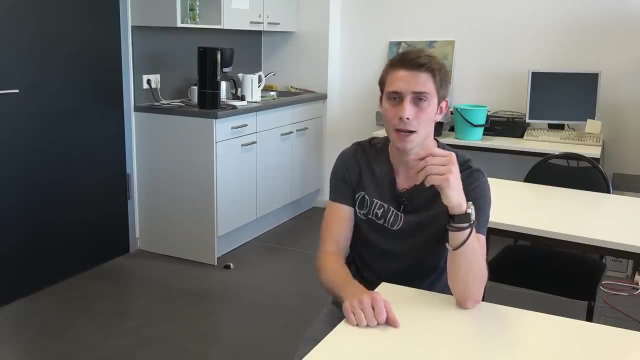 I'm so glad that I'm out of there. I couldn't bear listening to Professor Chattington anymore. This absolute math chat. Seriously, this guy is the peak of all unrigorousness, Andrew Chattington. 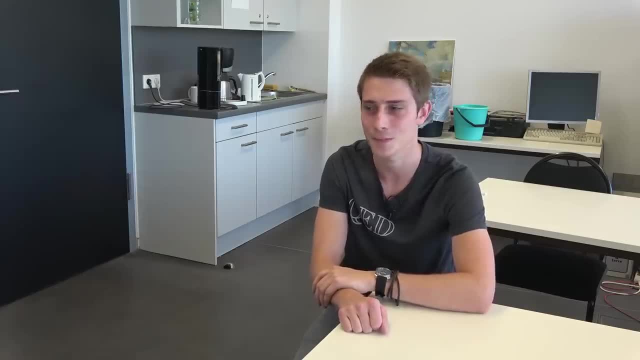 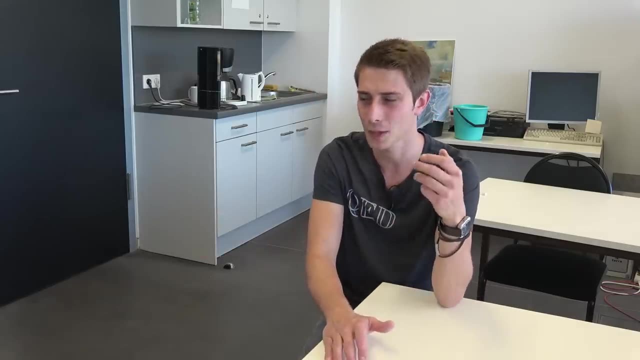 He's the enemy of all mankind. I hope I'm never going to become like him. I'm going to try and hone my math skills each and every day, be it in university or at home, And at home I can take a piece. 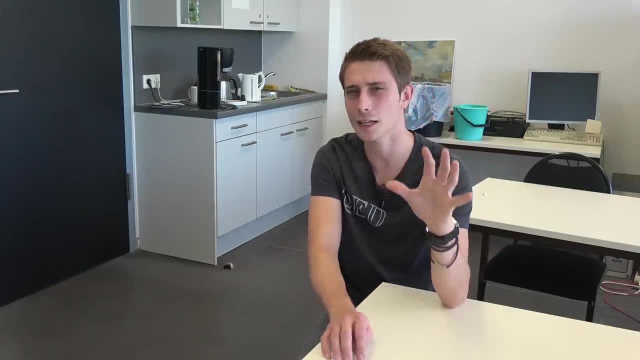 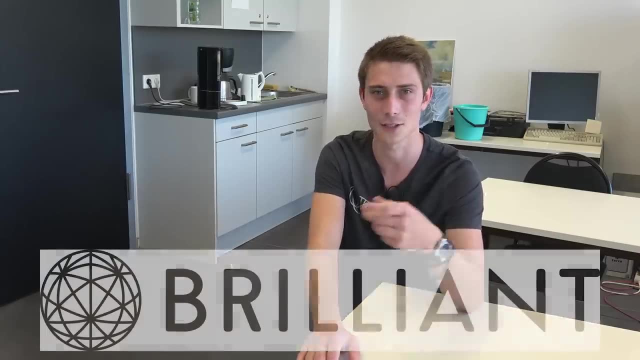 of paper and try out stuff for myself, But I like to use external tools from time to time, Be it Wikipedia, MathStack Exchange or Brilliantorg. By the way, this video has been sponsored by Brilliantorg. They really offer you a brilliant service. So, Brilliantorg. 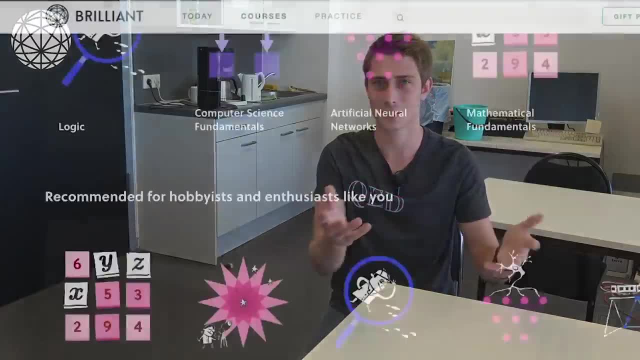 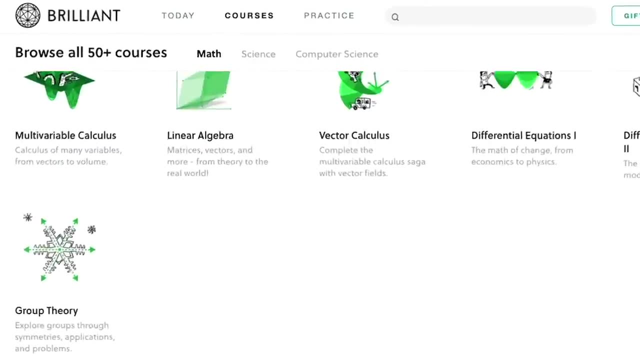 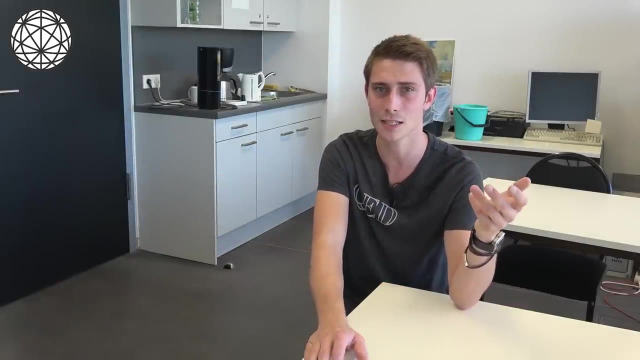 basically is an online learning platform. They have topics ranging from physics, mathematics, over to chemistry, everything, special relativity, analytic number theory, statistics whatsoever. They offer you such a wide variety of topics And the best thing is, you can learn actively by. 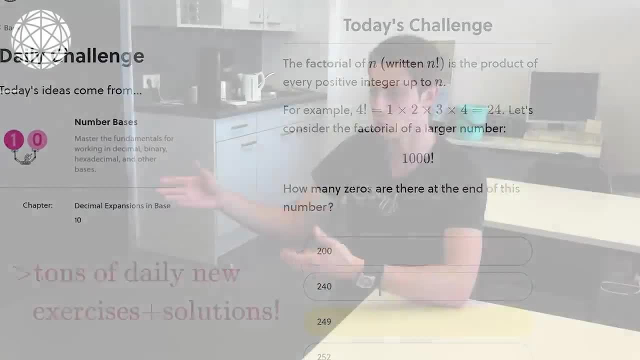 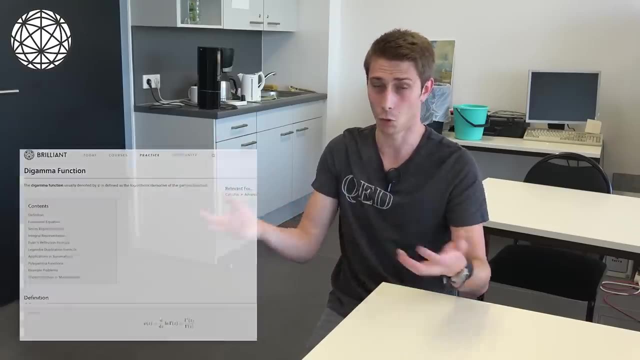 doing exercises on this page, Be it doing the exercise of the community- they even have their own community- or taking a look at their Wikipedia page and trying out stuff there. Or you can do the daily problems, for example, and try out a lot of different things there. It's absolutely. 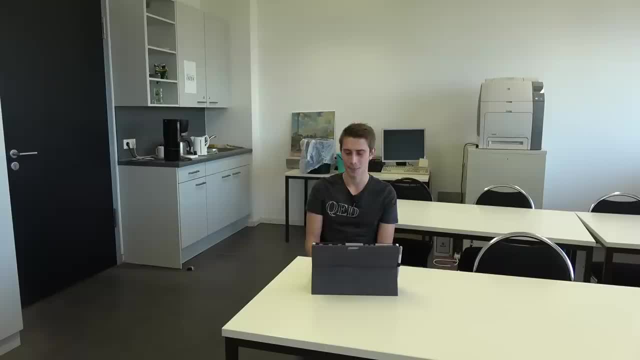 we're going to go ahead and expand it in a Taylor series centered at zero. But, Professor Chattington, even though the function is infinitely often differentiable, I agree on that- It is not analytical Meaning. we cannot turn it into a Taylor series. 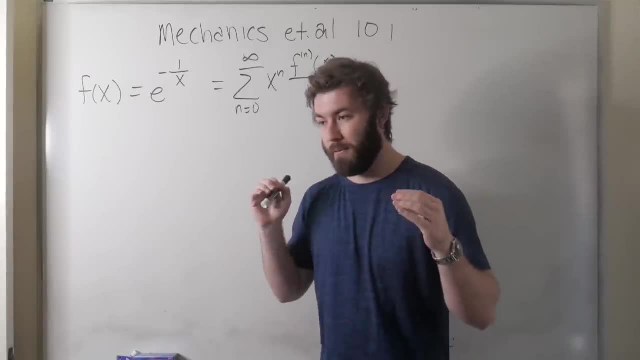 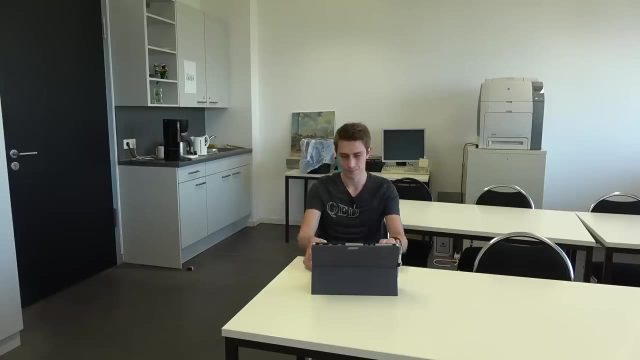 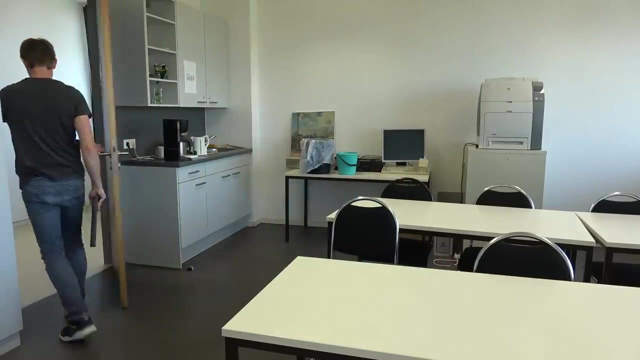 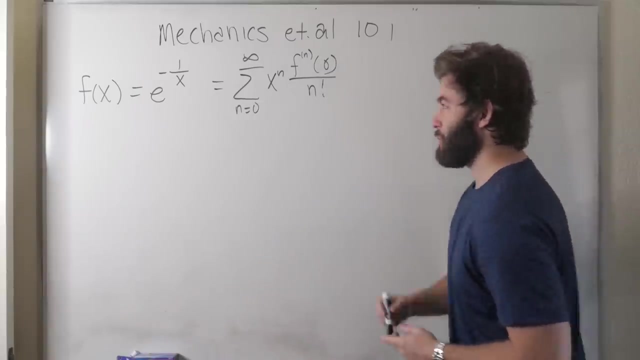 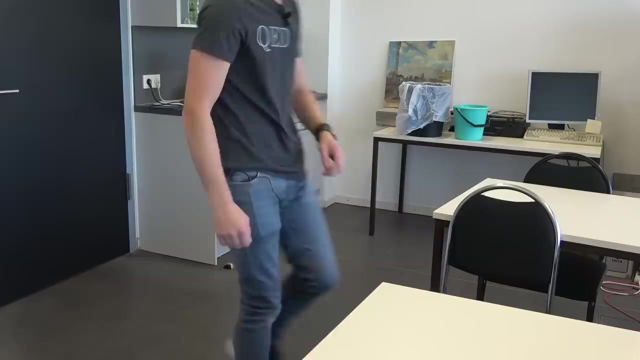 Even though it's infinitely differentiable. What are you even saying? Listen, if you have questions about the rigor of this class, you can leave. Please, I'm a head out. Okay, where were we? 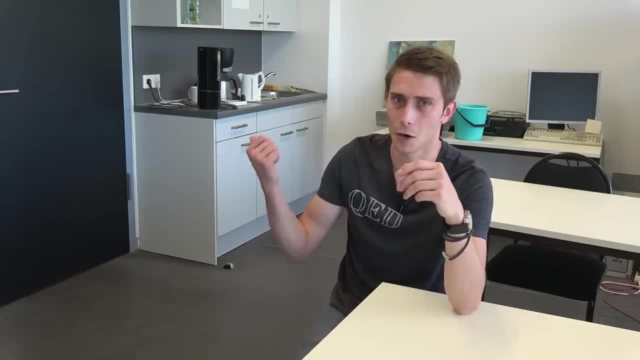 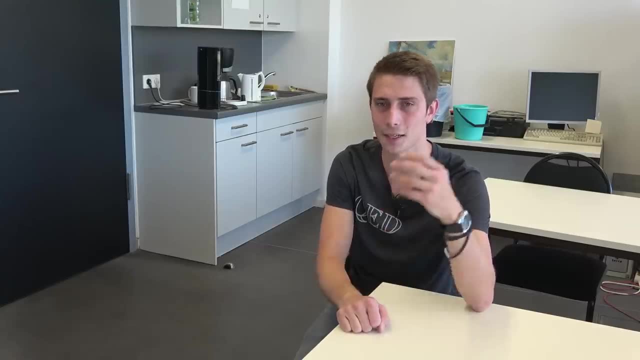 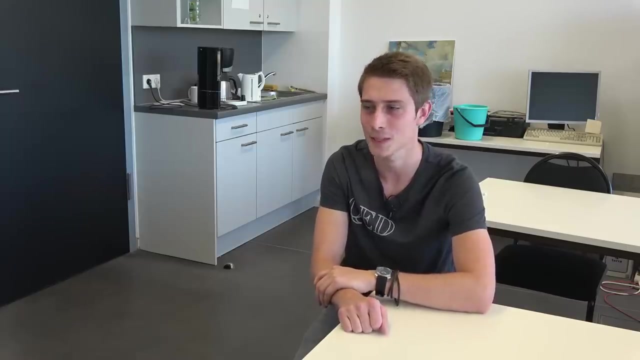 I'm so glad that I'm out of there. I couldn't bear listening to Professor Chattington anymore. This absolute math chat. Seriously, this guy is the peak of all unrigorousness. Andrew Chattington, He's the enemy of all mankind. 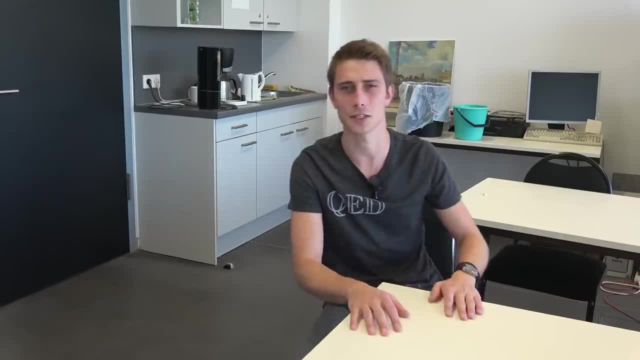 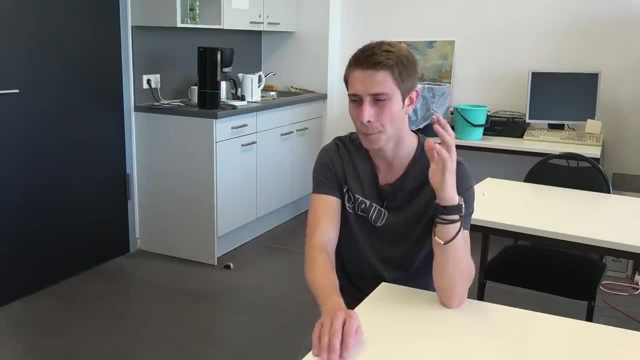 I hope I'm never going to become like him. I'm going to try and hone my math skills each and every day, be it in university or at home, And at home I can take a piece of paper and try out stuff for myself, But I like to use 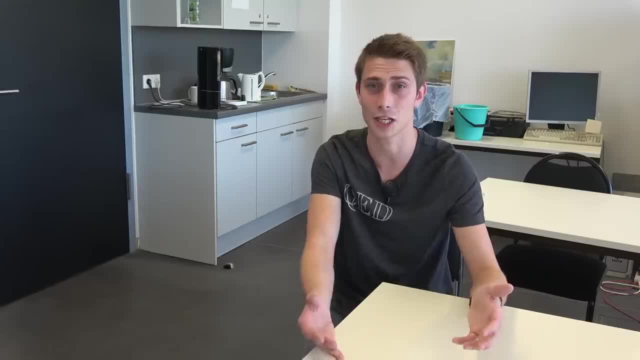 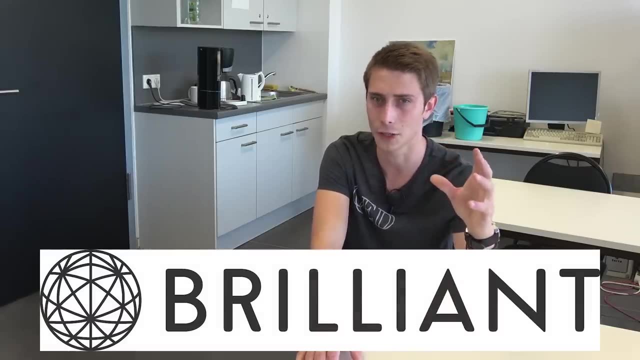 external tools from time to time, Be it Wikipedia, MathStack, Exchange or Brilliantorg. By the way, this video has been sponsored by Brilliantorg. They really offer you a brilliant service. So Brilliantorg, basically, is an online learning platform They have 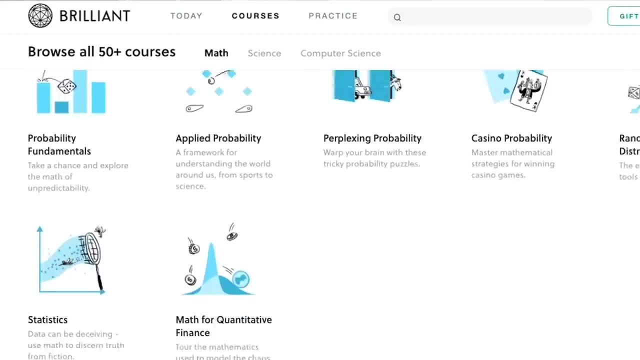 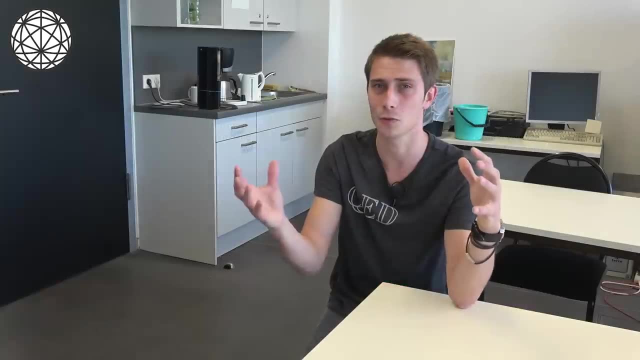 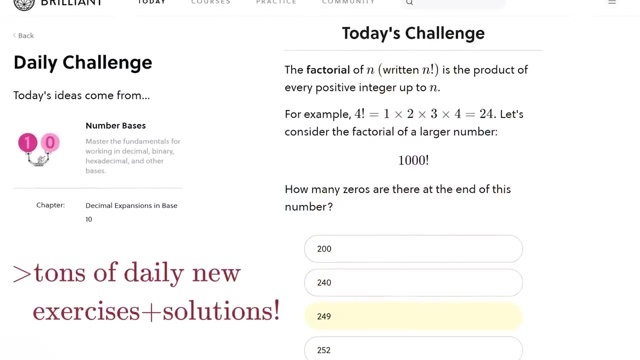 topics ranging from physics, mathematics, over to chemistry, everything, Special relativity, analytic number theory, statistics whatsoever. They offer you such a wide variety of topics And, the best thing is, you can learn actively by doing exercises on this page, Be it doing the exercise of the community. 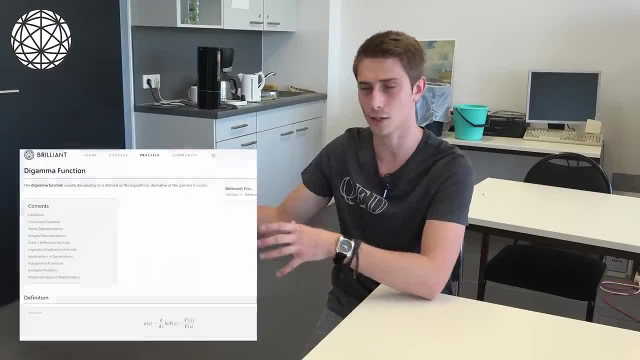 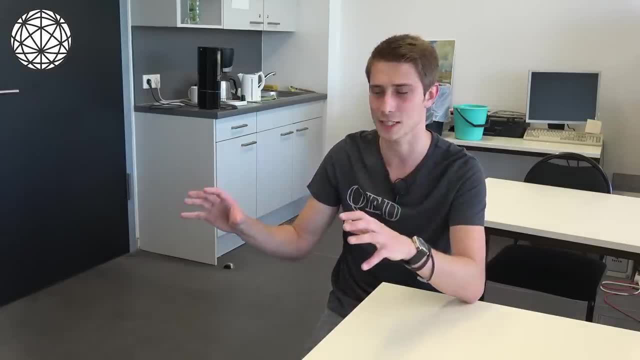 they even have their own community. or taking a look at their Wikipedia page and trying out stuff there. Or you can do the daily problems, for example, and try out a lot of different things there. It's absolutely amazing They have such a great repertoire of. 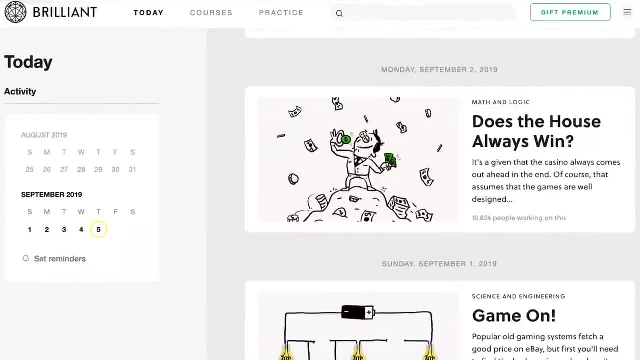 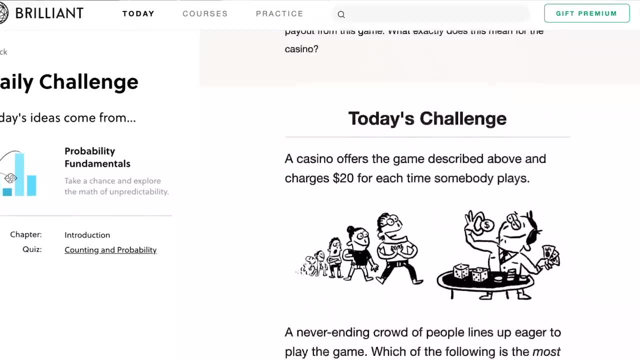 so many exercises. And the best thing is, even if you mess it up, even if you don't put in the right solution two or three times, you can take a look at the real solutions and maybe even by the community crafted recipes to get all the way down to the solution.